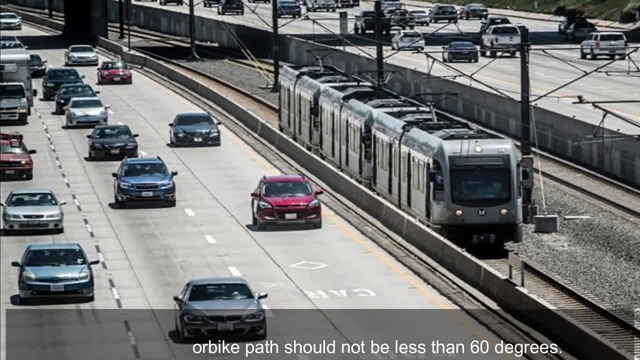 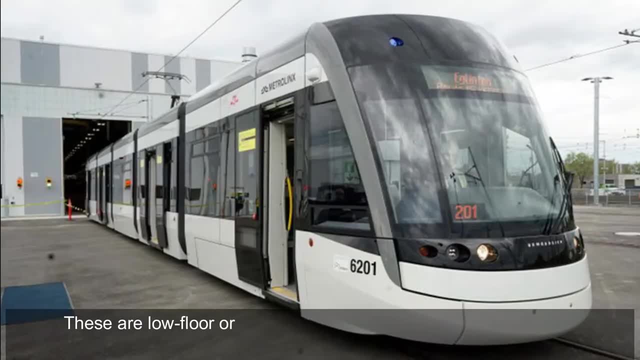 between tracks and motorbike path should not be less than 60 degrees. What are the components of a light rail transit system? Light rail transit vehicle? These are low floor or partially low floor vehicles with one or more independently rotating wheels instead of conventional solid 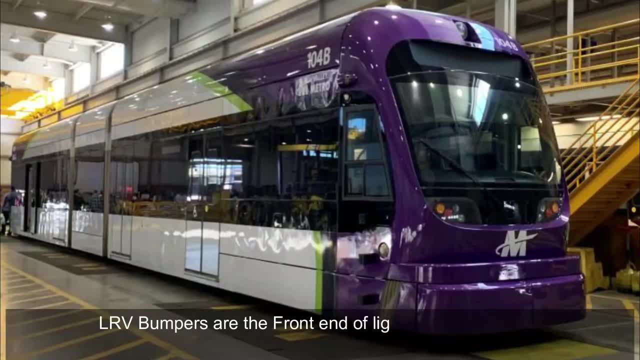 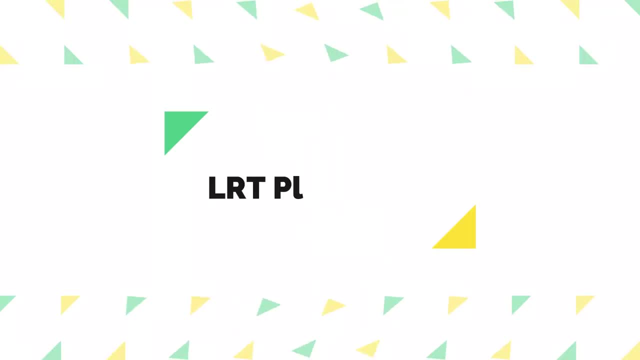 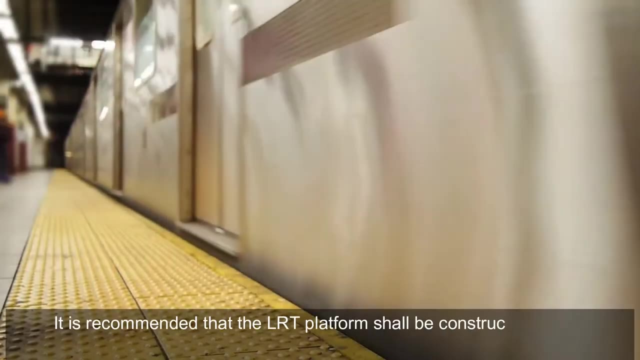 axles. LRV bumpers. LRV bumpers are the front end of light rail vehicles and they are designed around crash energy management, CEM principles, LRT platforms: LRT platforms are provided to the board and or a light from the trams. It is recommended that the LRT platform shall be constructed outside. 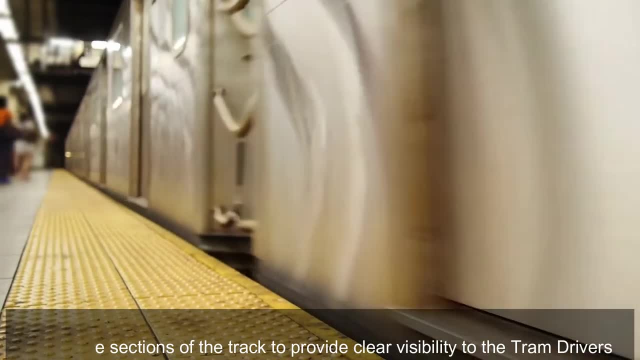 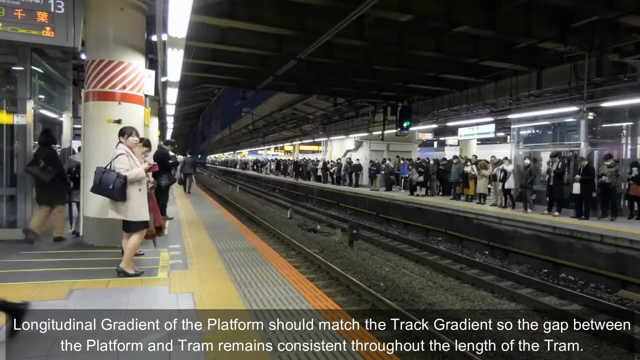 the curve sections of the track to provide clear visibility to the tram drivers. Longitudinal gradient of the platform should match the track gradient so the gap between the platform and the tram remains consistent throughout the length of the tram. What is the difference between LRT and? 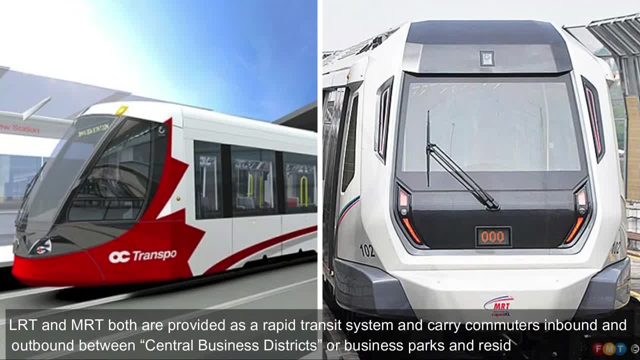 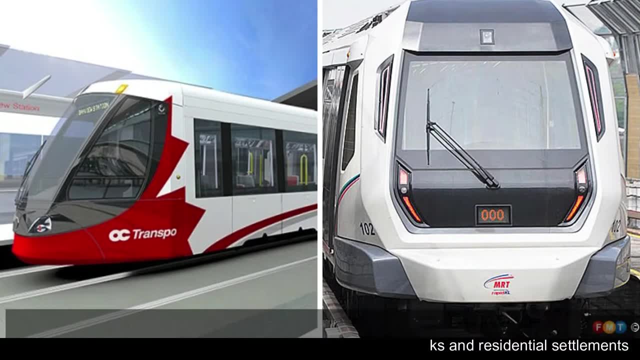 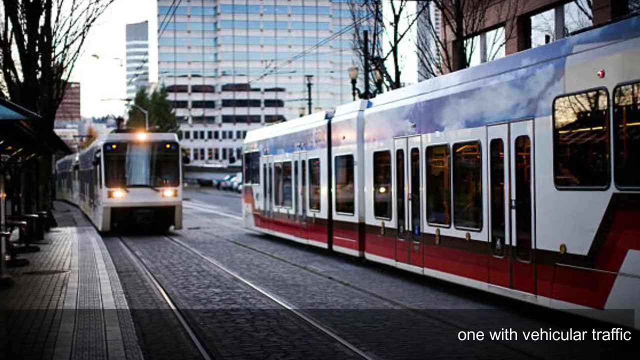 MRT. LRT and MRT. both are provided as a rapid transit system and carry commuters inbound and outbound between central business districts or business parks and residential settlements. Tracks LRT is plied in a combination of segregated zone and shared zone with vehicular traffic. 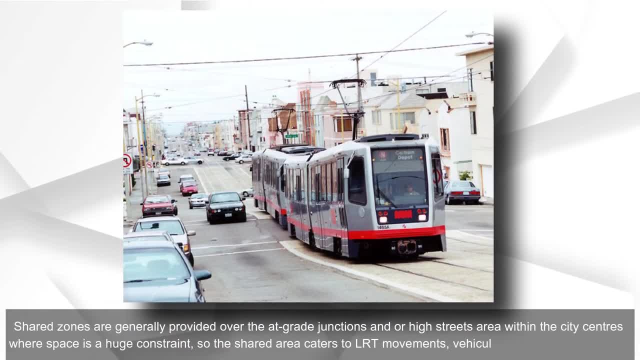 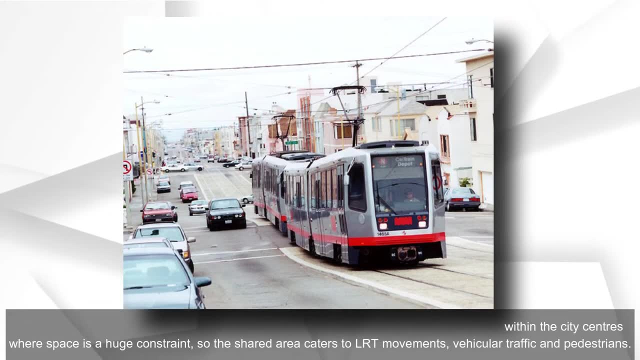 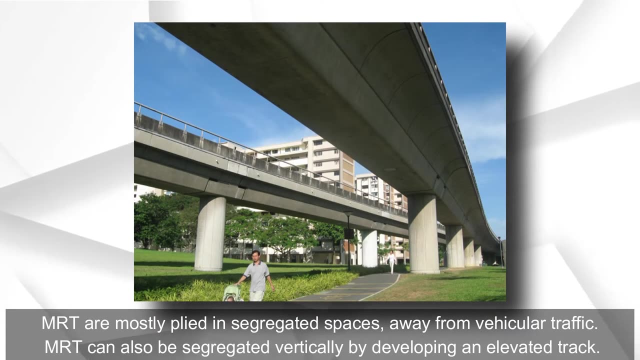 Shared zones are generally provided over the at-grade junctions and or high streets area within structures where space is a huge constraint. so the shared area caters to LRT movements, vehicular traffic and pedestrians. MRT are mostly plied in segregated spaces away from vehicular. 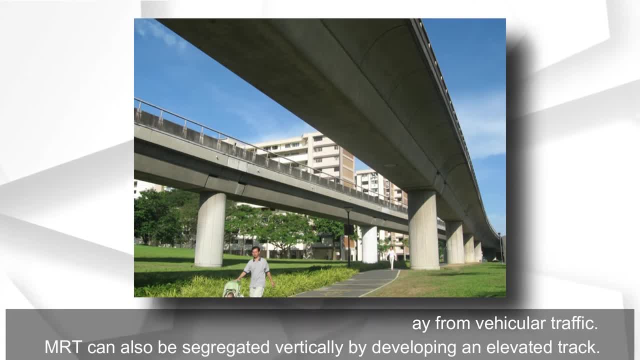 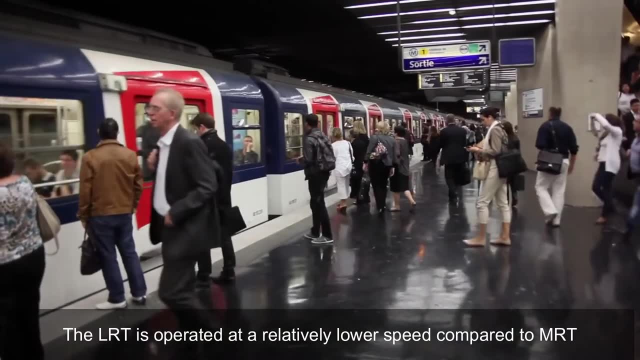 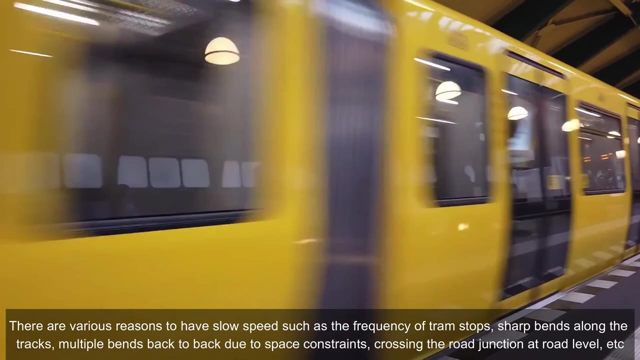 traffic. MRT can also be segregated vertically by developing an elevated track Speed of LRT and MRT. The LRT is operated at a relatively lower speed compared to MRT. There are various reasons to have slow speeds, such as the frequency of tram stops, sharp bends along the tracks. 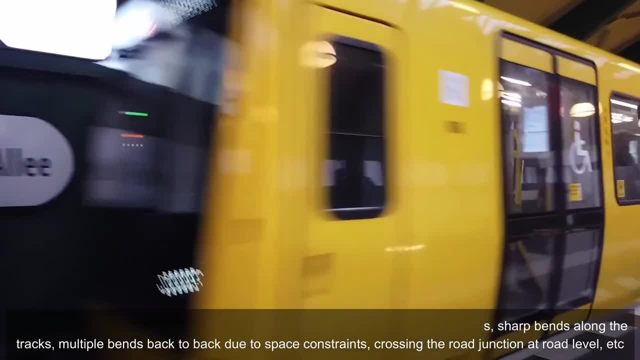 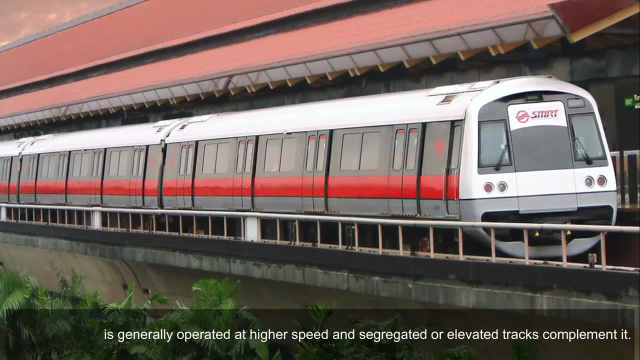 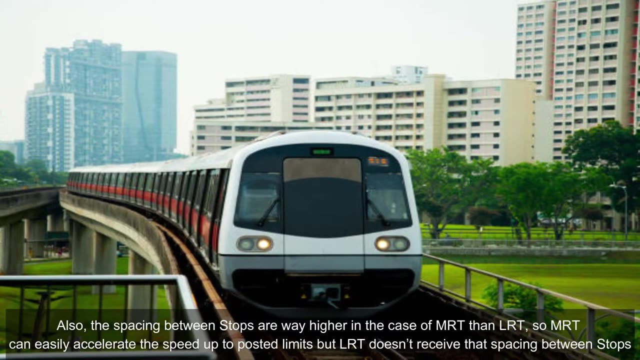 multiple bends back to back due to space constraints, crossing the road junction at road level, etc. However, MRT is generally operated at higher speed and segregated or elevated tracks complemented. Also, the spacing between stops are way higher in the case of MRT than LRT. so 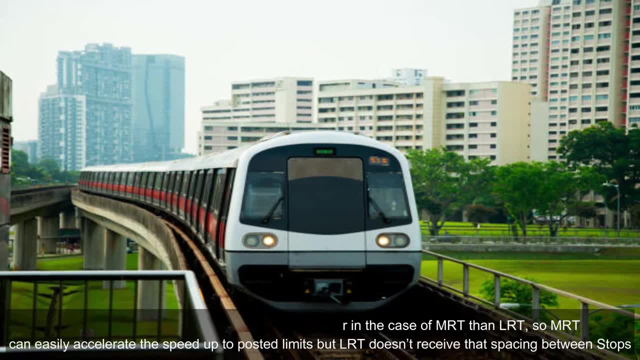 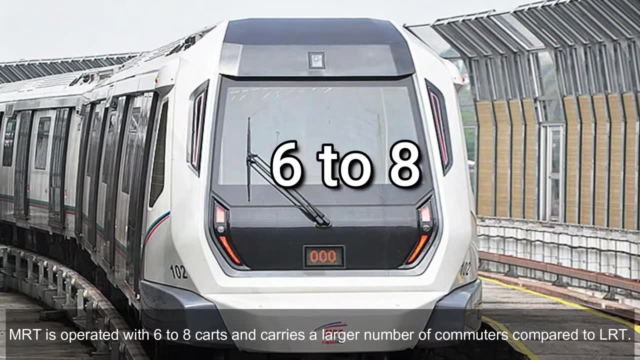 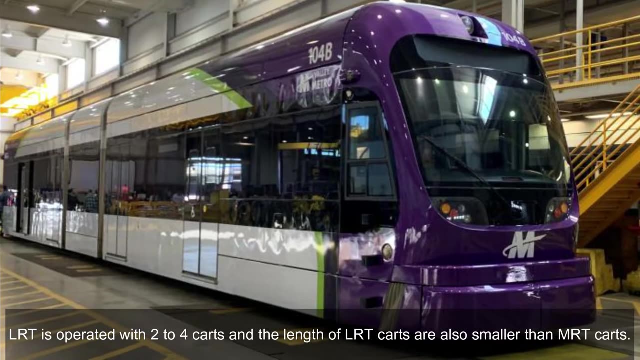 MRT can easily accelerate the speed up to posted limits, but LRT doesn't receive that spacing between stops. Number of carts: MRT is operated with six to eight carts and carries a larger number of commuters compared to LRT. LRT is operated with two to four carts and the length of LRT carts are: 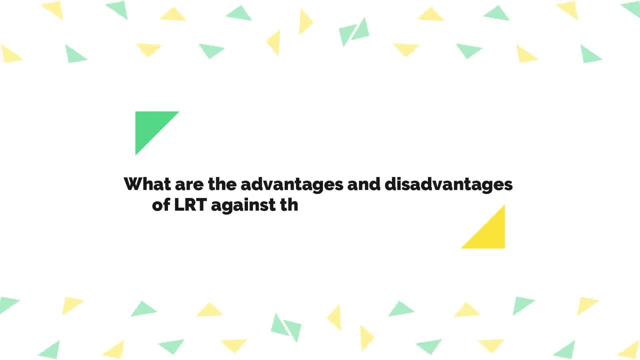 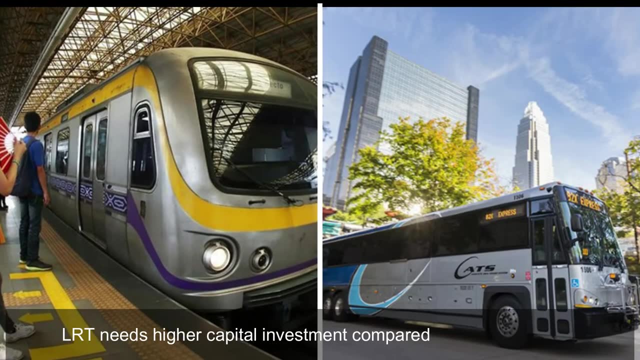 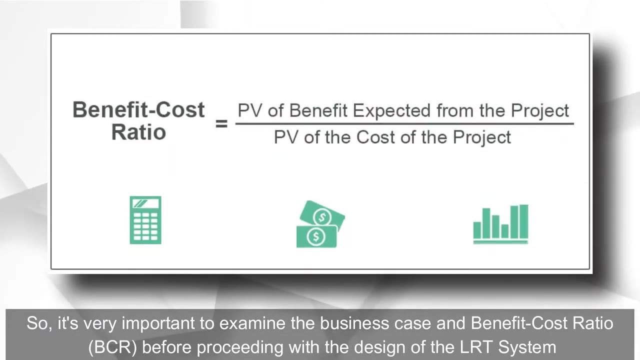 also smaller than MRT carts. What are the advantages and disadvantages of LRT against the buses and slash for MRT Construction cost? LRT needs higher capital investment compared to the bus system, So it's very important to examine the business case and benefit cost ratio- BCR- before proceeding. 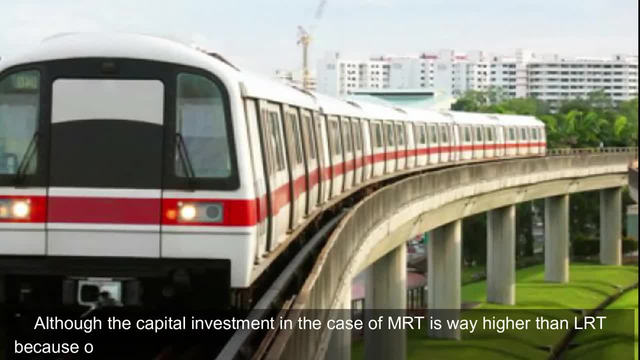 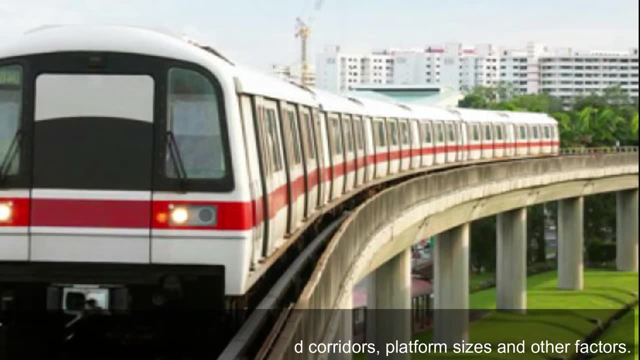 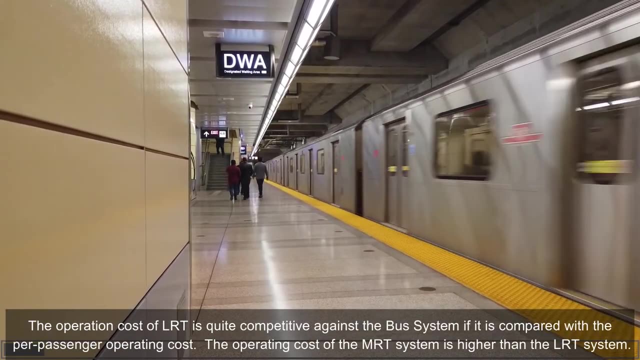 with the design of the LRT system, Although the capital investment in the case of MRT is way higher than LRT because of its long lengths, dedicated corridors, platform sizes and other factors. Operation cost: The operation cost of LRT is quite competitive against the bus system if it is compared with the per passenger operating cost. 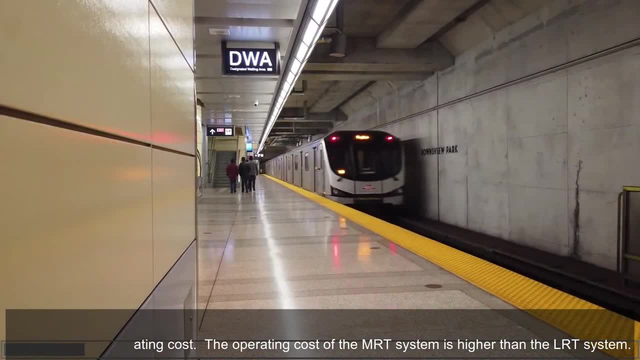 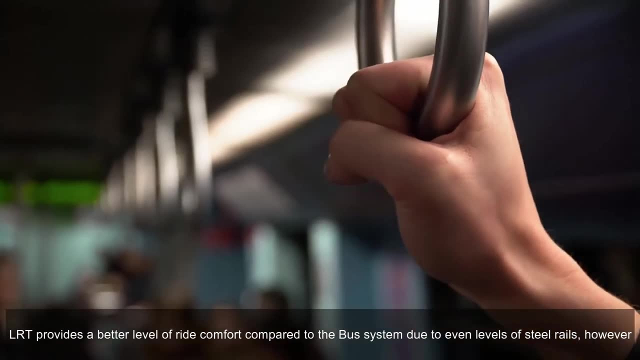 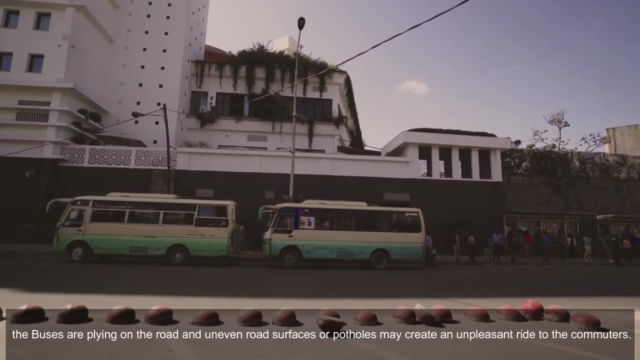 The operating cost of the MRT system is higher than the LRT system. Ride comfort LRT provides a better level of ride comfort compared to the bus system, due to even levels of steel rails. however, The buses are plying on the road and uneven road surfaces or potholes may create an unpleasant ride. 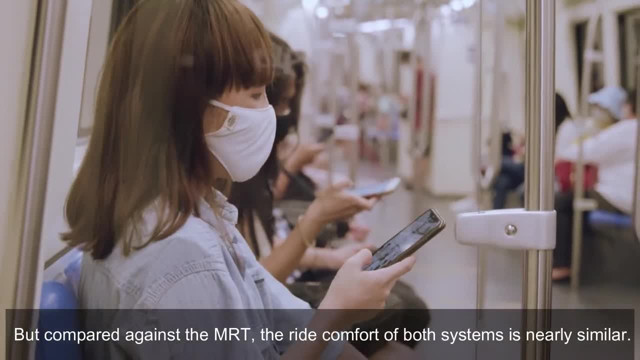 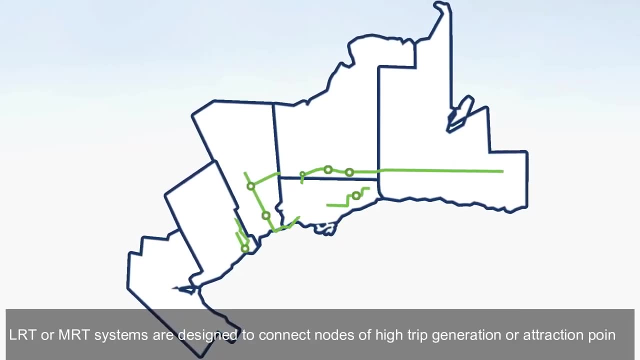 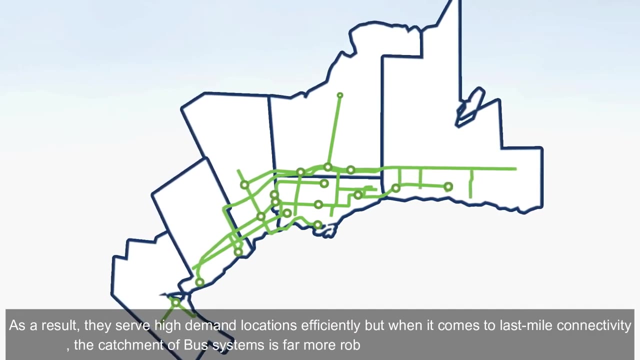 to the commuters, But compared against the MRT, the ride comfort of both systems is nearly similar Last mile connectivity. LRT or MRT systems are designed to connect nodes of high trip generation or attraction points. As a result, they serve high demand locations efficiently, but when it 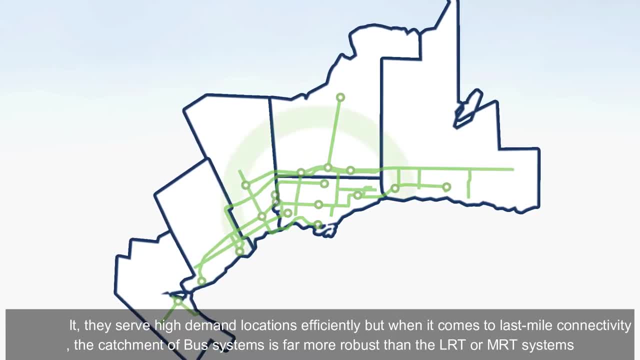 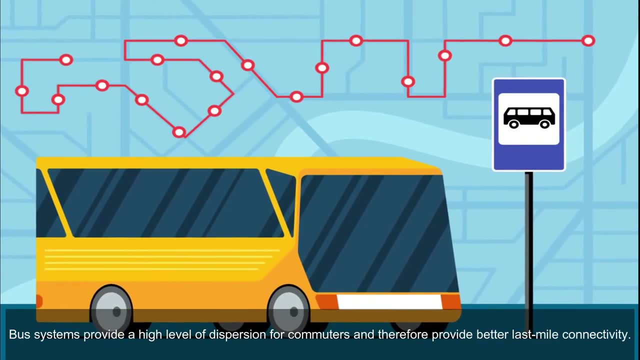 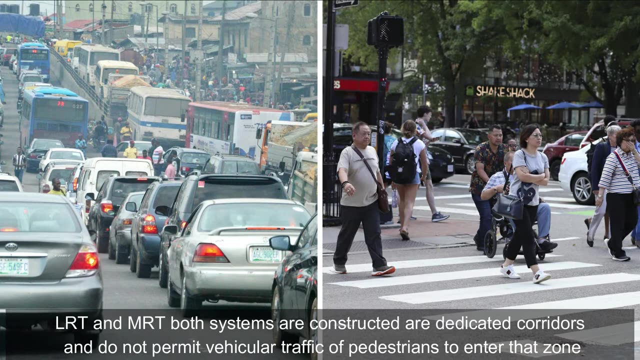 comes to last mile connectivity, the catchment of bus systems is far more robust than the LRT or MRT systems. Bus systems provide a high level of dispersion for commuters and therefore provide better last mile connectivity Safety. LRT and MRT: both systems are constructed or dedicated corridors. 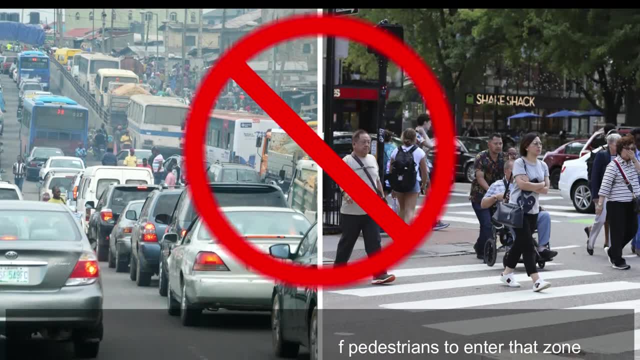 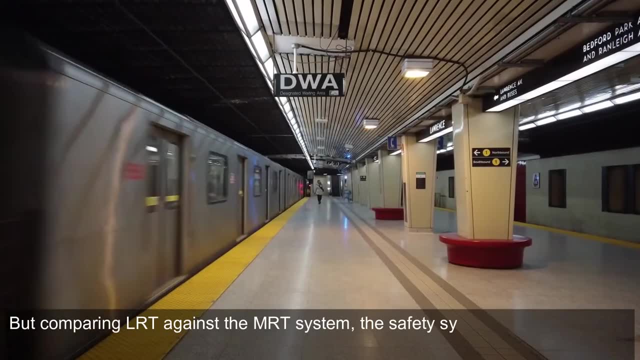 and do not permit vehicular traffic of pedestrians to enter that zone. As a result, the safety of LRT or MRT systems are way higher than bus systems. But comparing LRT against the MRT system, the safety system of MRT is higher than the LRT system because the LRT system is more stable than the MRT system. 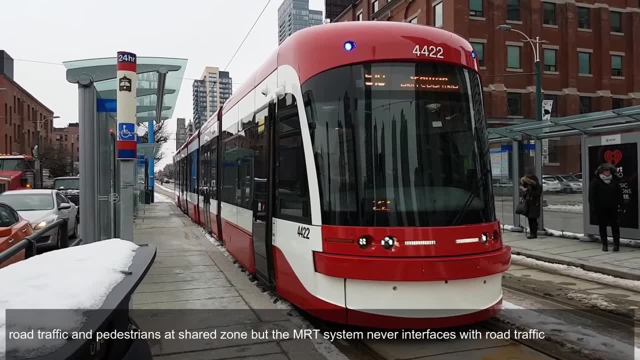 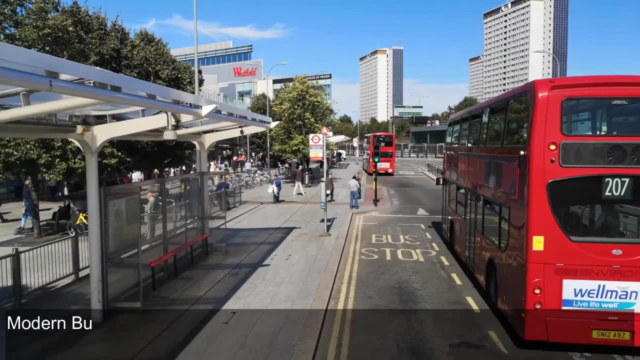 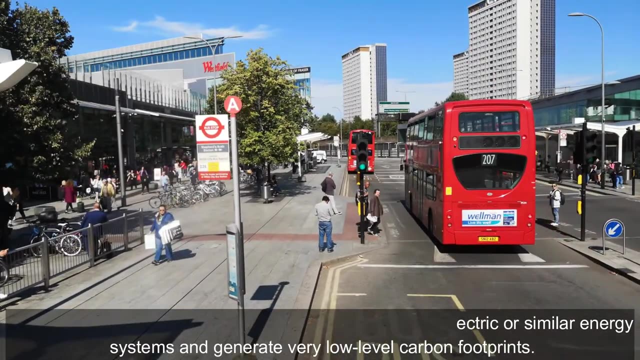 LRT system sometimes interacts with road traffic and pedestrians at shared zone, but the MRT system never interfaces with road traffic or pedestrians. Environmental impacts: Modern buses are generally operated by using CNG or electric or similar energy systems and generate very low level carbon footprints, But MRT and LRT are operated by propulsion power from an overhead distribution.